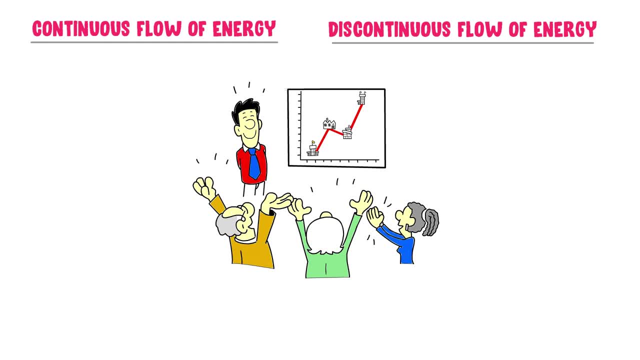 theory which no one is teaching us in the school or college course. Remember that continuous flow of energy happens in our daily life, while discontinuous flow of energy happens at microscopic level. Firstly, let me teach you the concept of continuous flow of energy. Consider a ball. 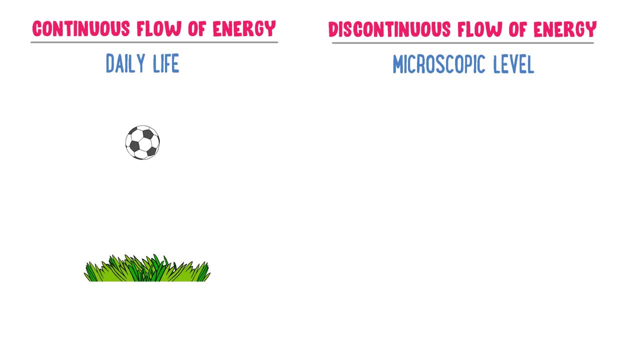 present at certain height above the ground, We know that it possesses potential energy. Now, when this ball falls toward the ground, its potential energy is converted to kinetic energy. Here comes the most important question: Can I change the value of potential energy or kinetic energy of this ball? Well, the answer is yes. It is in my control. I can. 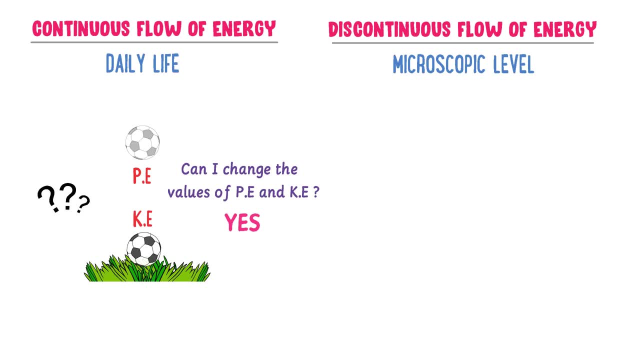 change its value. The next question is: How can I change the value of potential energy, or kinetic energy of this ball? Well, the answer is yes, It is in my control. I can change its value. How can I change its value? Well, it is simple. Change the height of the ball to desired level. 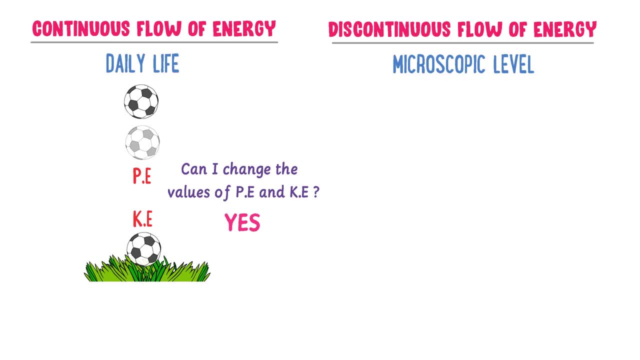 and the values of potential energy and kinetic energy would be changed. It means that it is in my control to change the values of potential energy and kinetic energy to 5 Joule, 6 Joule, 7 Joule, 8 Joule, etc. Therefore we say that in this case, energy 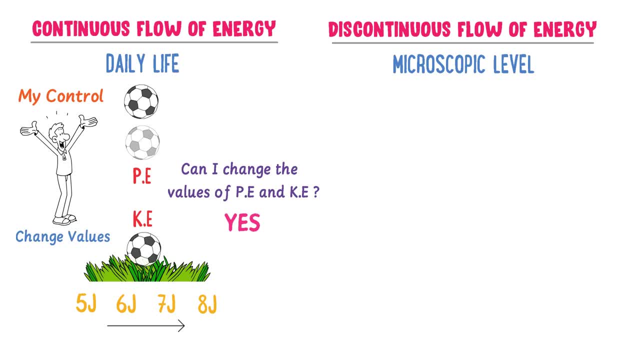 flow and continuous way, or flow of energy is continuous because I can control it or I can change it. Now, coming to the concept of discontinuous flow of energy, According to Bohr's atomic model, electron can reside in different energy levels, like first energy level, second energy. 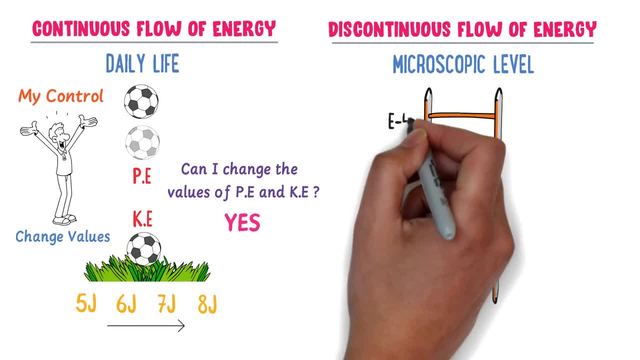 level, third energy level and fourth energy level, like strips of a ladder. Now consider electron at highest energy level, fourth energy level. Let this electron jumps from fourth energy level to third energy level. When it jumps from higher energy level to lower energy level, it loses our radiate energy. Let it loses 15 Joule energy. Secondly, this: 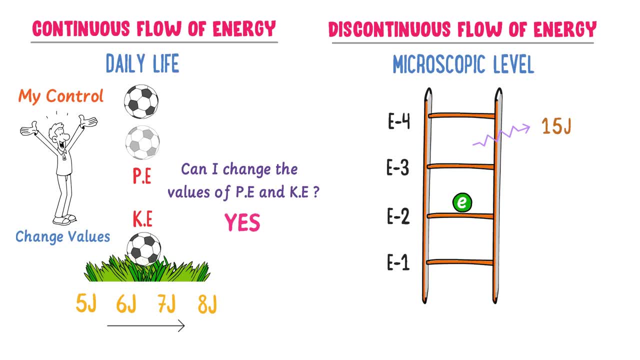 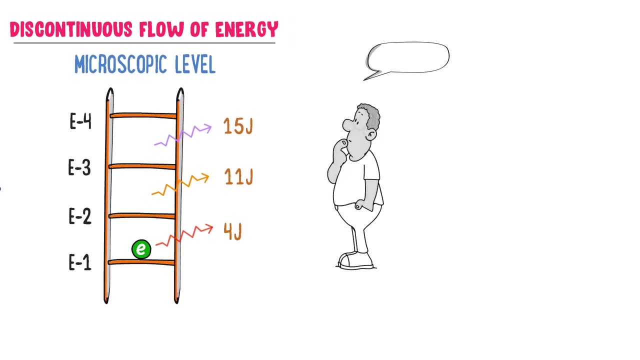 electron jumps from third energy level to second energy level and also loses 11 Joule energy. Thirdly, it jumps from second energy level to first energy level and it loses 4 Joule energy. Now listen carefully. I am interested that when an electron jumps from 4th energy 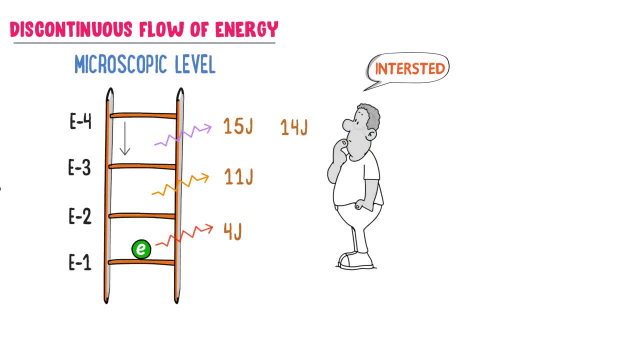 level to 3rd energy level, it should lose only 14 Joule energy. When it jumps from third energy level to second energy level, it should lose only 13 Joule energy, And when it jumps from second energy level, it should lose only 12 J energy. I mean the flow of energy must be continuous. 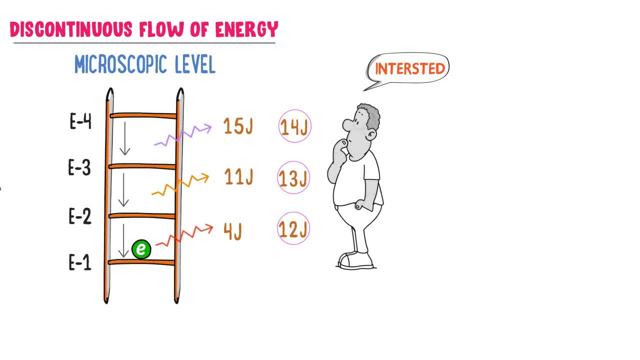 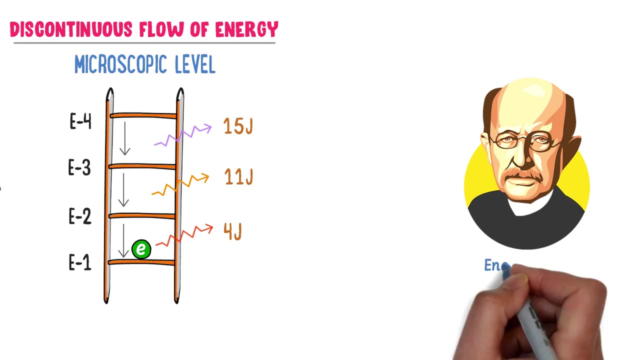 14 J, 13 J, 12 J, according to my wishes. Now let me ask you: is it possible? Well, here comes Max Planck, Baba, that it is not possible and it is totally wrong. Energy flow in a discontinuous manner at microscopic level. 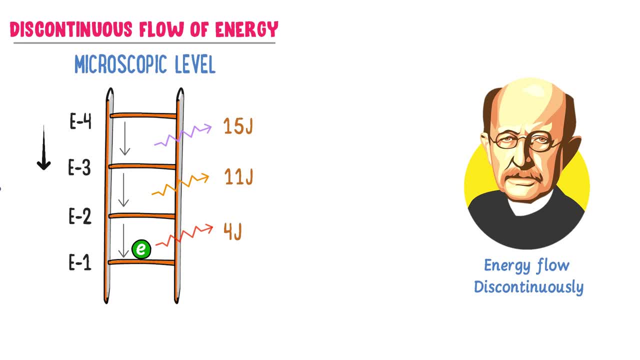 Planck Baba says that when electron jumps from 4th energy level to 3rd energy level, it lose fixed amount of energy. 15 J energy and the form of discrete wave packet like this are just like a chocolate packet. Note it down that the word discrete means individually, separate or unique. 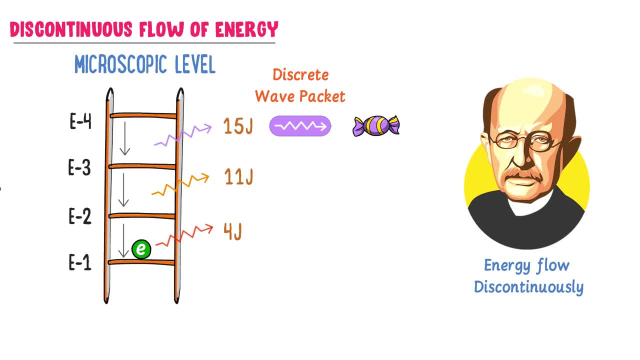 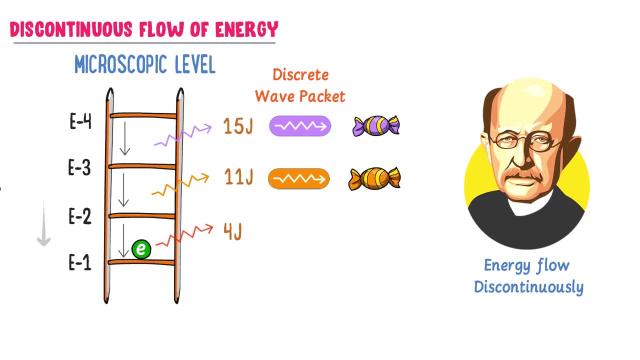 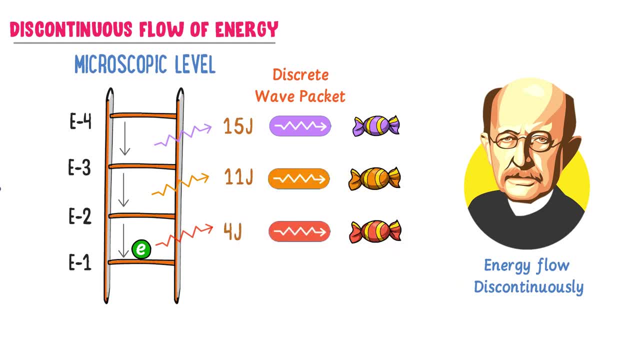 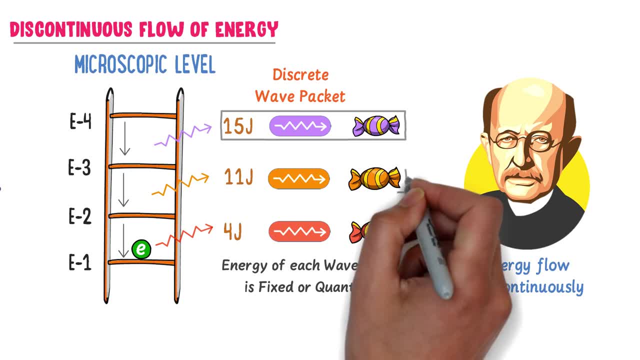 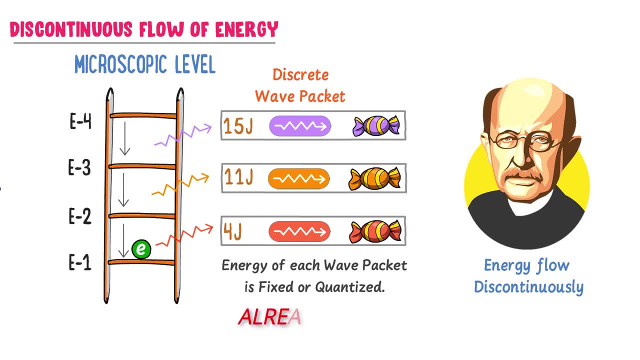 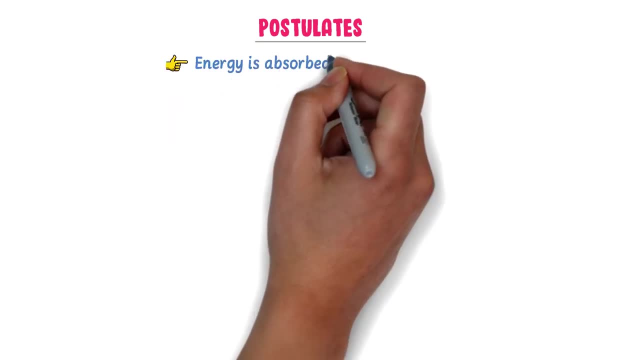 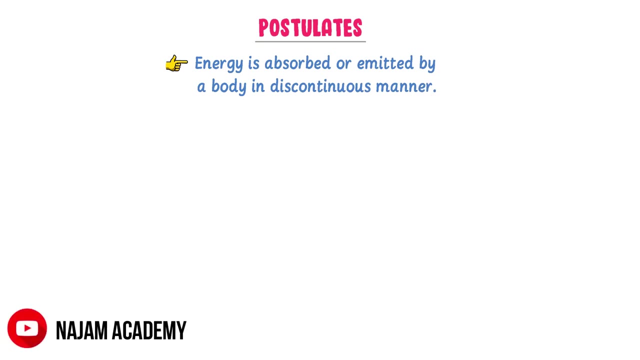 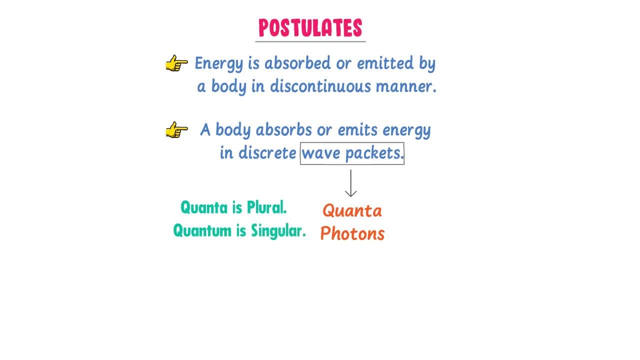 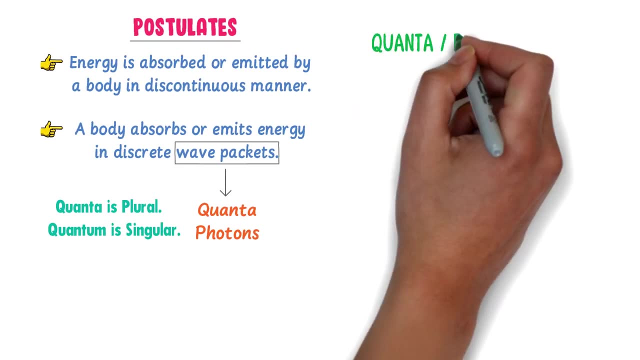 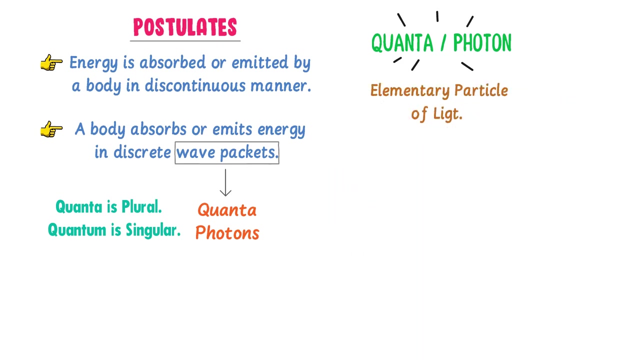 3., 4., 5. hovering Airlines, 6. for all the relationships, 5. balance wave packets. Now, what is Quanta or Photon? Well, photon or quanta is the elementary particle of light, or we can say it is the basic unit. 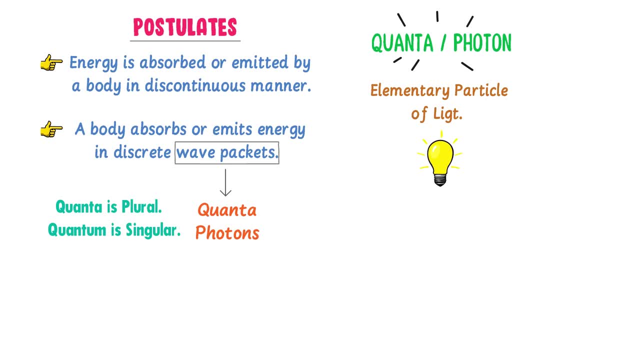 of light. It means that every light or radiation is made up of billions or trillions of photons. Photons are nothing, but they are made up of electric field and magnetic field. They have no charge, they have no rest mass and they travel at the speed of light. 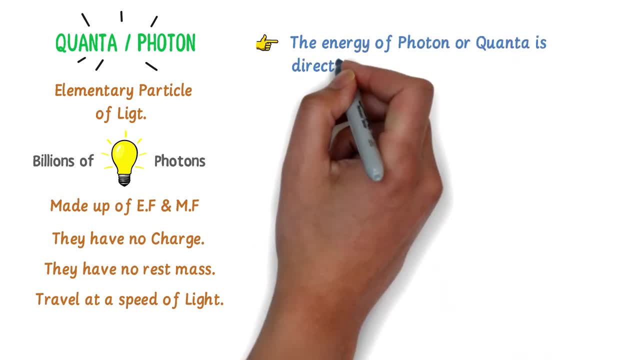 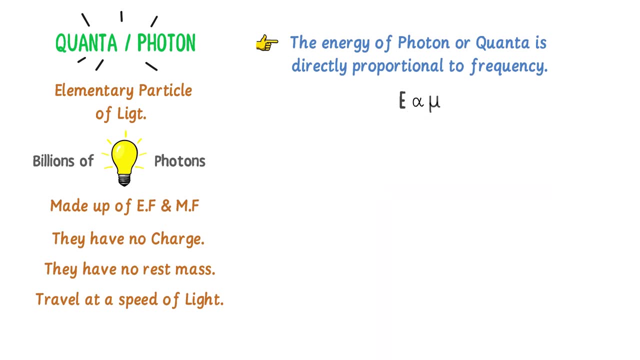 Thirdly, the energy of protons, or quanta, is directly proportional to the frequency. E is directly proportional to mu. For example, consider blue photon and red photon. The frequency of blue photon is high and the frequency of red photon is low. 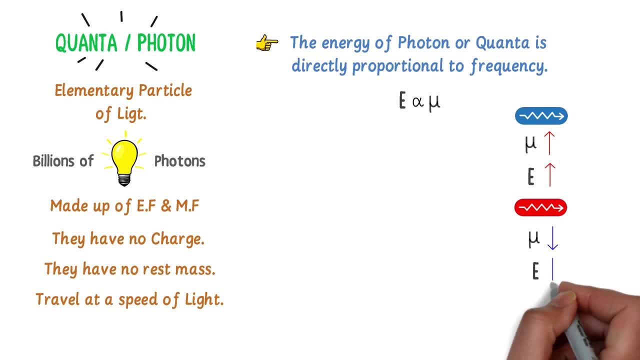 So the energy of blue photon is high and that of red photon is low. Now to eliminate the sign of proportionality, we put h, which is known as Planck's constant and its value is 6.626, into 10 to the power negative 34 joule second.